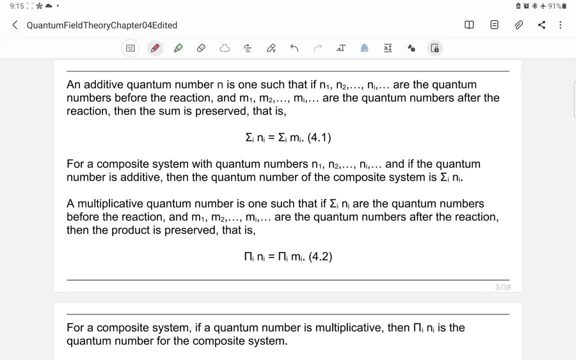 n is one such that if you have particular quantum numbers, say n1 into ni, and that's before reaction, and if you have different quantum numbers after the reaction, then the sum will just be the same, even though they are not, I mean the same initially and at the final state. So the sum should be the same for 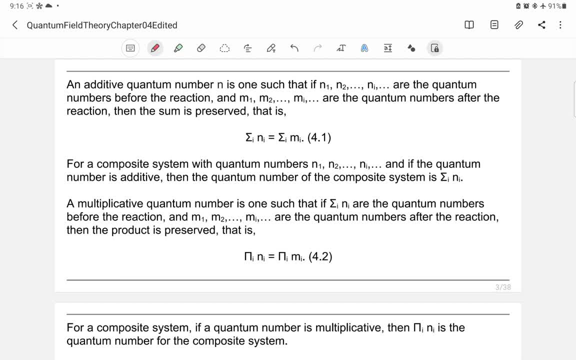 any reaction. There are also multiplicative quantum numbers, such that if you have quantum numbers in its initial state or, for example, before collision or scattering or decay, then the multiplication of these quantum numbers at the beginning would also be the same in the final state, The product or the. 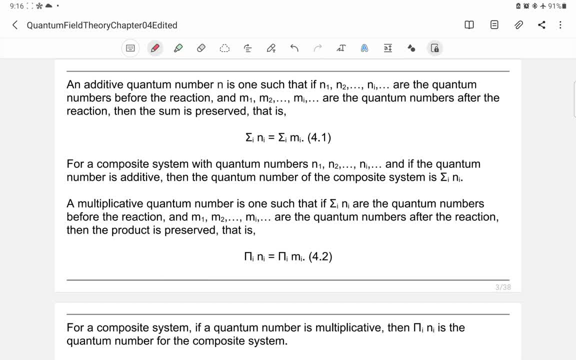 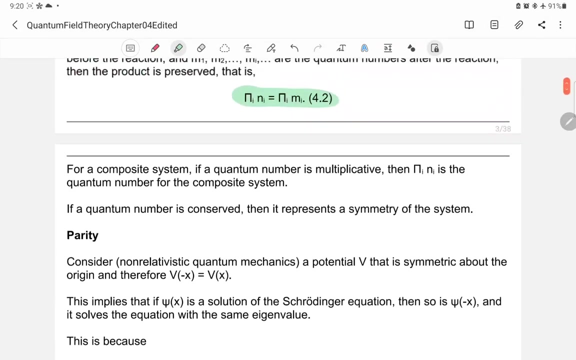 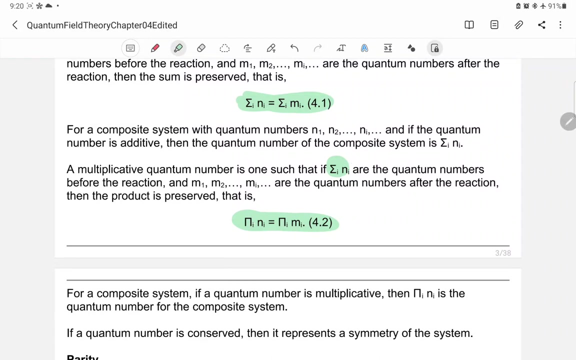 multiplication of those quantum numbers. Sorry, this is supposed to be product, not sum. So anyway, remember this For the active quantum numbers and for the multiplicative quantum numbers. Here we go…. Ah, Here we go…. By the way, err, I I missed something here. this is supposed to be this. 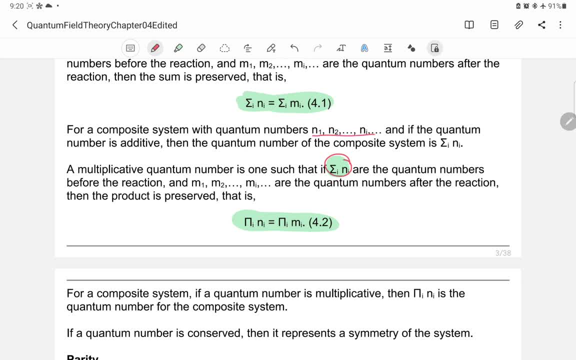 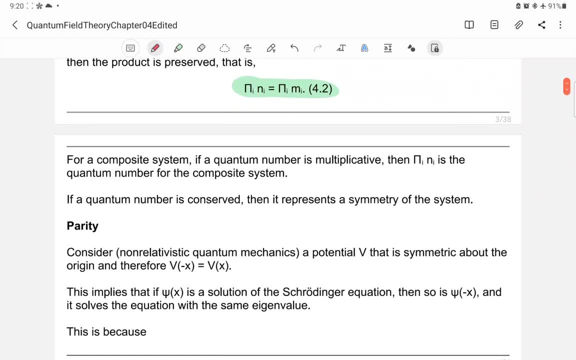 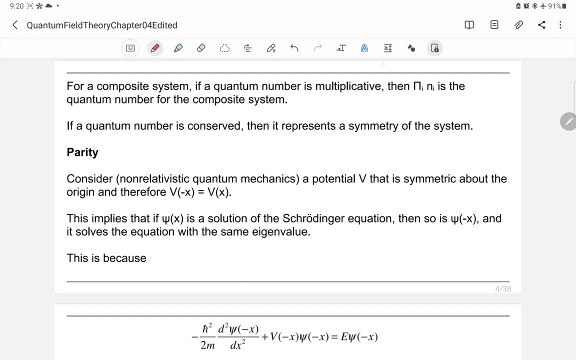 one here. It's supposed to be this. Okay, so for a composite system, if a quantum number is multiplicative, then the product of the quantum numbers is the quantum number of the composite system. and also, if a quantum number is conserved, then it represents a symmetry of the system. now we'll start with the first symmetry, and this is: 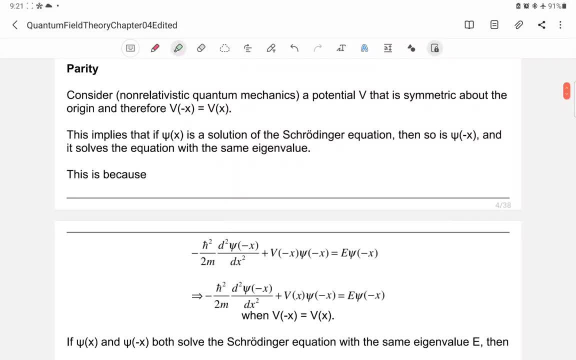 just the parity. so, for example, in non relativistic quantum mechanics, consider a potential be that is symmetric about the origin, and so you will have this one. this implies that if you have a wave function, psi X- to be a solution, the Schrodinger equation- then this is also a solution together with this, so it solves the equation with the same. 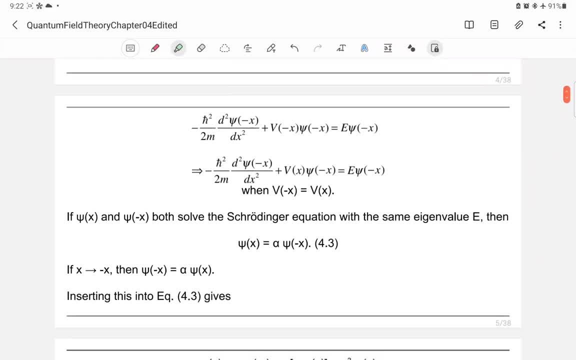 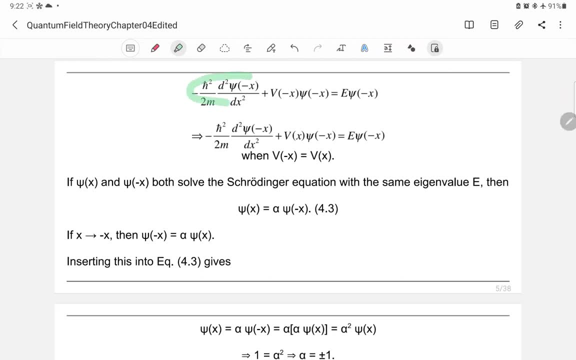 eigenvalue, because when you look at the Schrodinger equation here, it's just just the Schrodinger equation. however, when your potential is has this symmetry, then it's just the Schrodinger equation, still the same. so therefore, you can write your this wave function. I mean, you can write this wave function in terms: 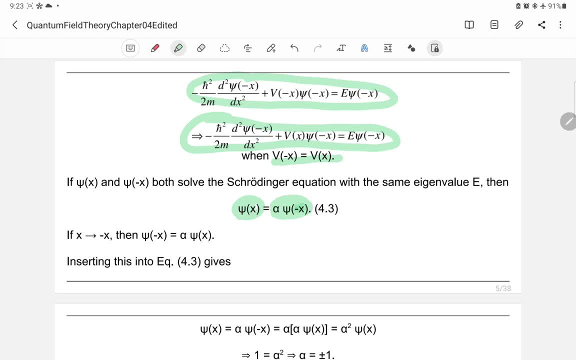 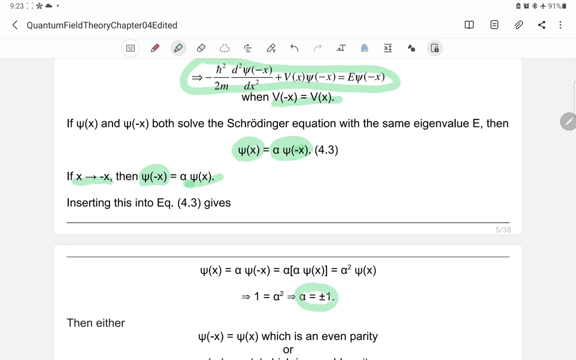 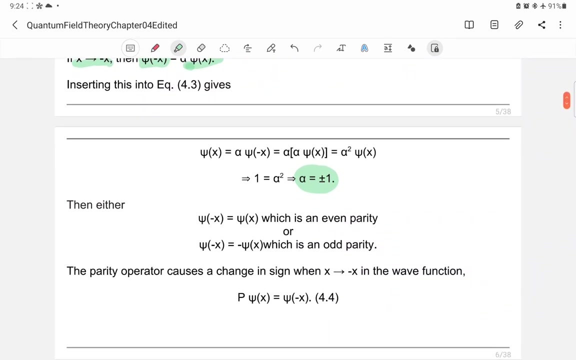 of this one here, and so if you transform X to negative X, then your wave function of negative X would also be alpha times your original wave function. so if you do that, you can get the eigenvalue alpha, which is just equal to 1 and negative 1, so this means that you have parity, that 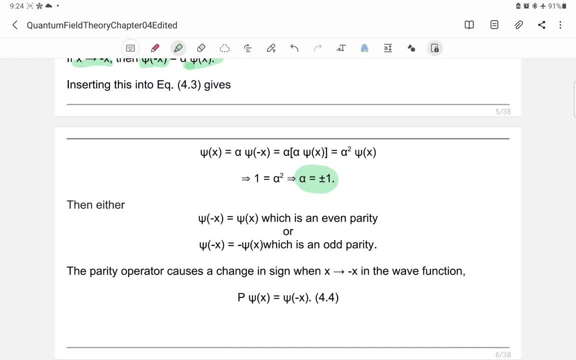 could be an even parity or an odd parity. so if your wave function would be transform like this, then you have an even parity, and if you have a wave function that transforms like this, and it should be an odd parity. the parity of rater causes the change in sign when X is transformed into negative. 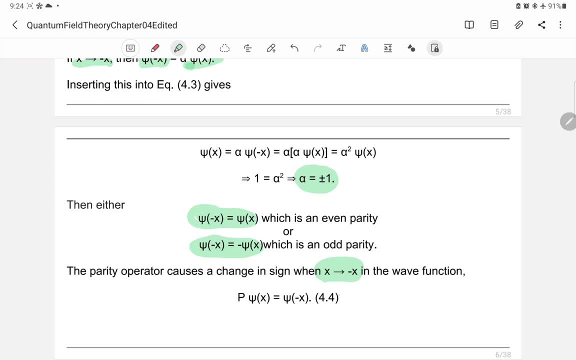 X in the wave function. in general it should be spaced, but in this discussion is just one directional and we just consider the space that's on the x-axis. so you take a wave function and then you apply a parity operator and this one is the result of that. it's just the side, but your space becomes. 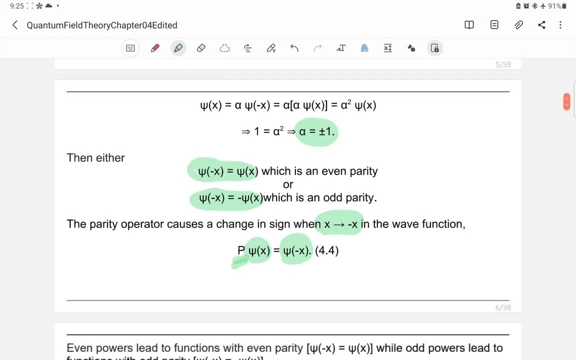 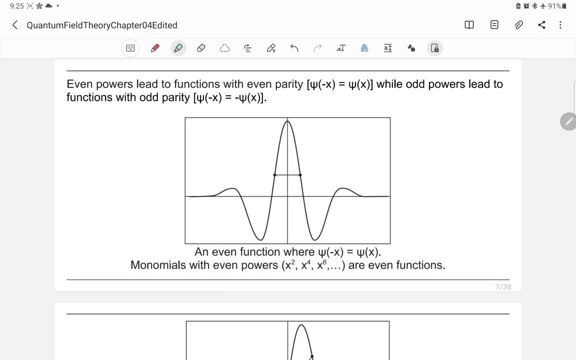 negative even powers lead to functions with even parity- this one while add powers lead to functions with odd parity and that one, so an even function where your sine negative X is equal to psi X. you have this kind of symmetry. if you flip in this case, in just for this case, if you flip on this axis, you would get: 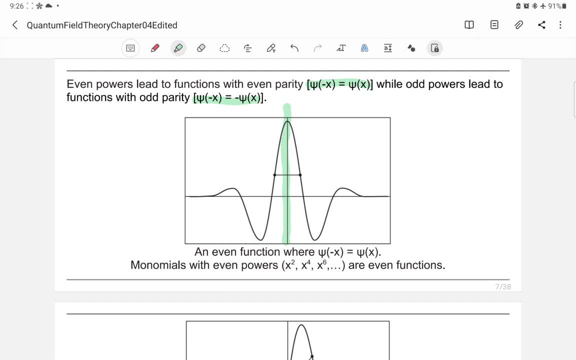 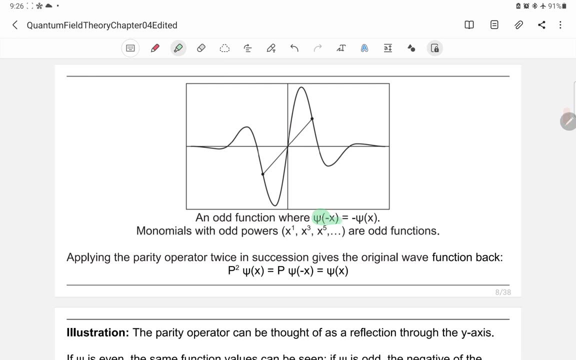 the same form of the way. flip about this axis here and for an odd part, an odd function, where this is the behavior. these are monomers with odd powers. say, for example, X to the first power, X cube X to the fifth, and so on. if you flip this, this figure here, 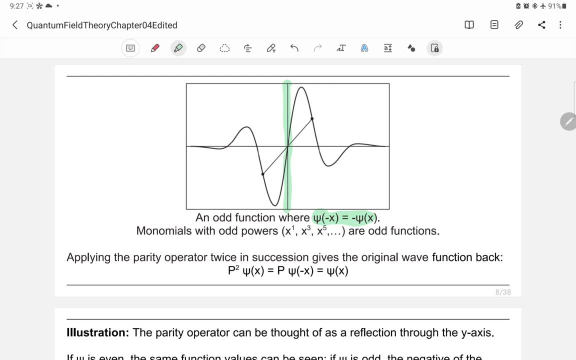 then the wave function will not coincide with each other, although they are. are if you, if you flip this, are, if you, if you flip this, this one here about this axis, then this would look like this: this particular frame, this would look like that and you will have an even evenости, certainstatheze, or an even. 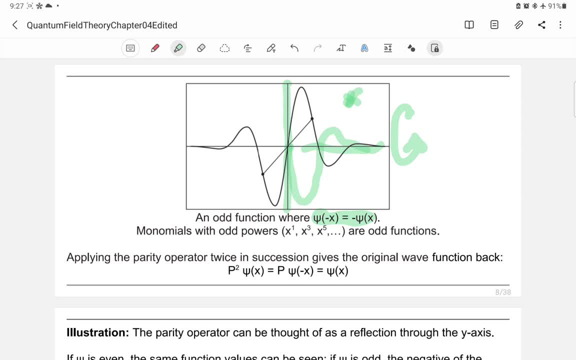 boundary term already. there will be alốno why they do. they are like that, the j понимаю case, but severely more powering. is there something wave function? but in this case it will not coincide with each other wherever axis that you flip, like this, for example, or here: 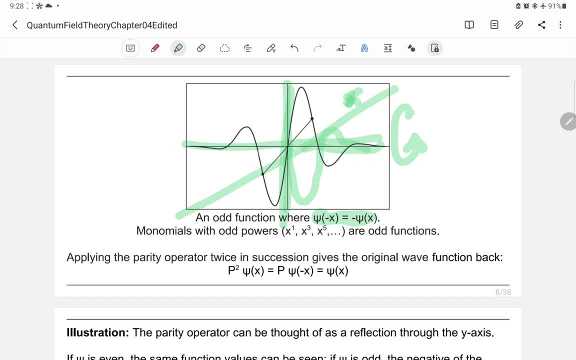 and even in this axis it will not. so that's it, that's for anyway. you can just um, you can be sure of that. when you have odd powers, if they are monomials without powers, then there are add functions and that if you have a function that is just composed. 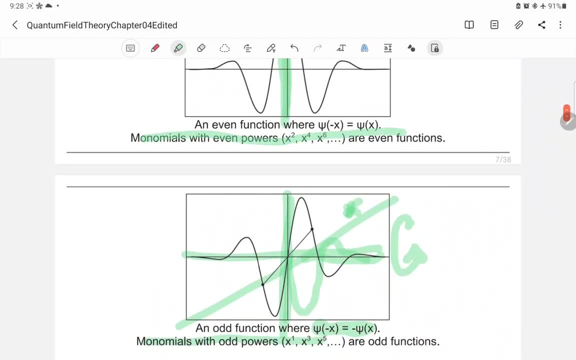 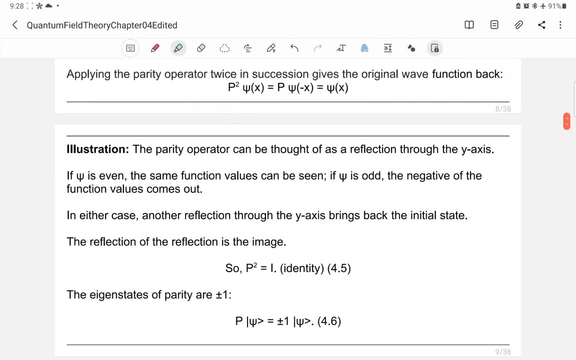 of even powers, of uh monomials with even powers, then that is an even function. applying the parity operator twice in succession gives the origin wave function back here. in this particular case the parity operator can be thought of as a reflection through the y-axis. so parity symmetry in a symmetry with what we call parity is: 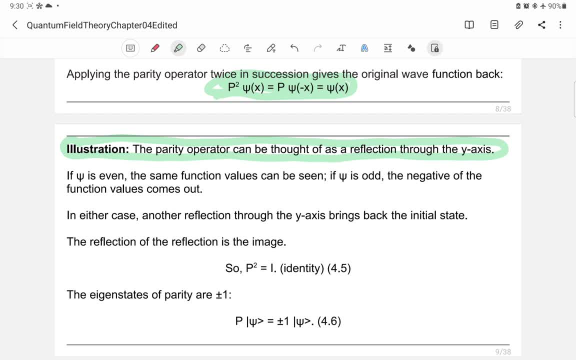 dealing with space, so it deals with space. so if we invert the space, then you would have that parity going on. so if psi is even the same, function values can be seen. if high is odd, the negative of the function, the negative of the function values. 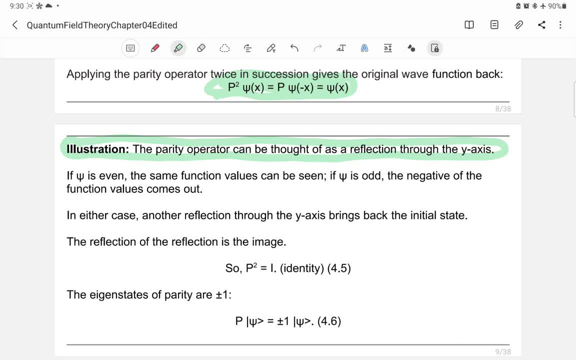 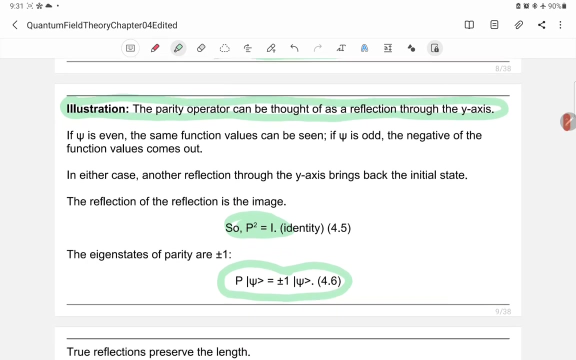 comes out. So in either case, another reflection through the y-axis brings back the initial state. So if you operate the parity twice, you will get an identity. The eigenstates of parity are plus minus one here, So that's the eigenvalues. I mean the eigenvalues are. 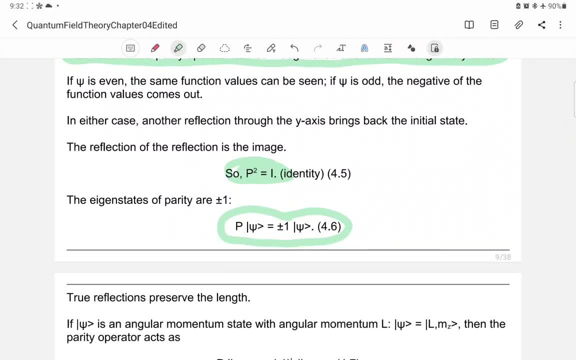 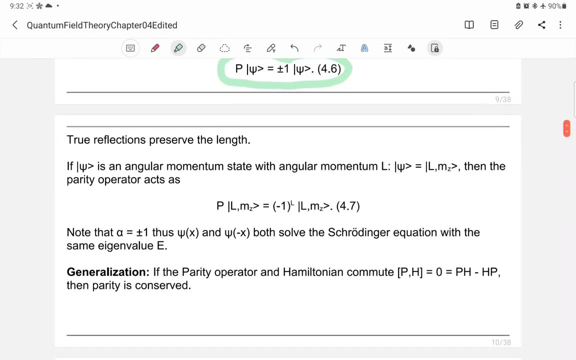 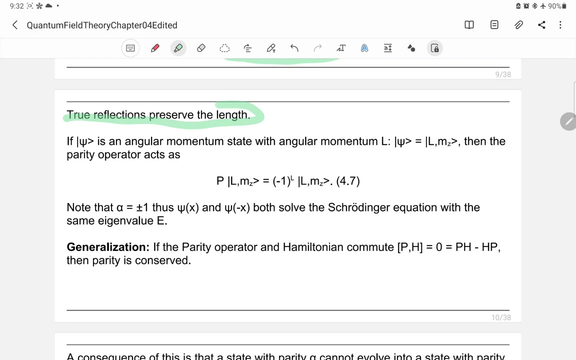 one minus one. Then you have the eigenstates just the positive or negative of the original one. True reflections preserve the length If it's just a reflection. Now, if your wave function psi is an angular momentum state, with angular momentum L here, 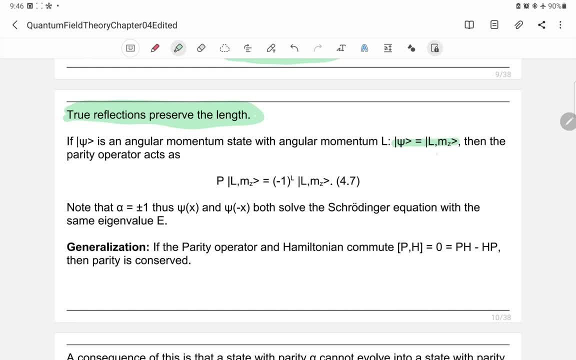 your state is written this way: If you would review your quantum mechanics, then the parity operator acts on that as this one. Note that alpha alpha here could just be positive or minus one. So your psi x and psi negative x would have to be solutions of the Schrodinger. 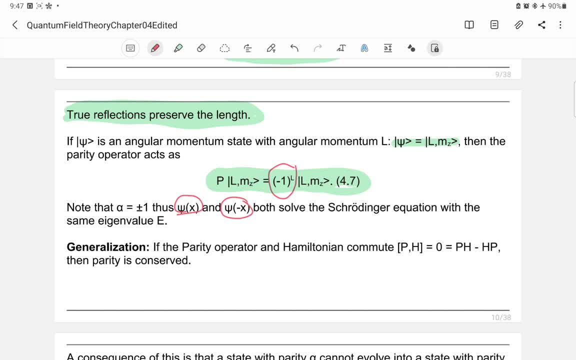 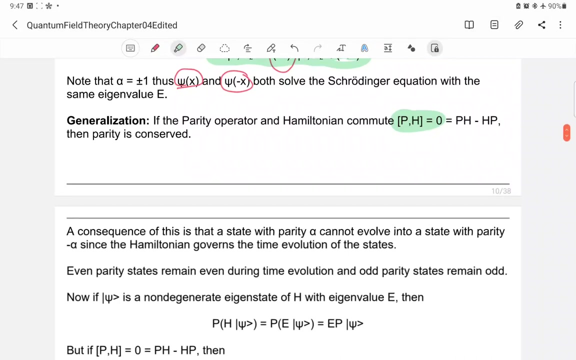 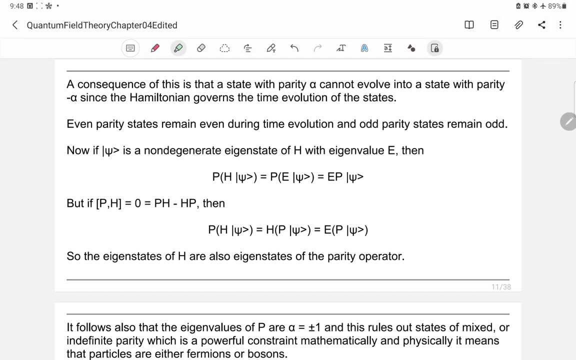 both would have to be solutions of the Schrodinger equation. It would be the same eigenvalue in general If the parity operator and Hamiltonian commute. So if they commute, then parity is conserved. A consequence of this is that the state with parity alpha cannot evolve into a state with alpha. 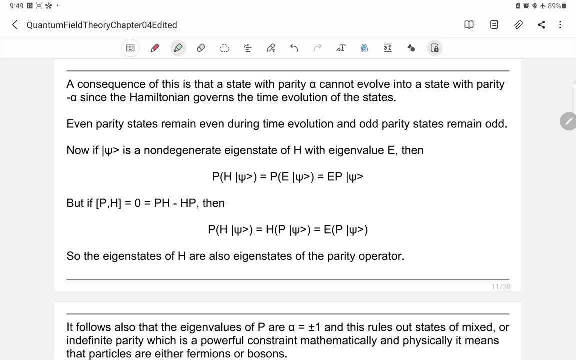 to a state with parity negative alpha, since the hamiltonian governs the time evolution of the states. so even parity remains even and odd parity remains during time evolution. so if you look at this, if considering a wave function that is non-degenerate eigenstate of h or hamiltonian, 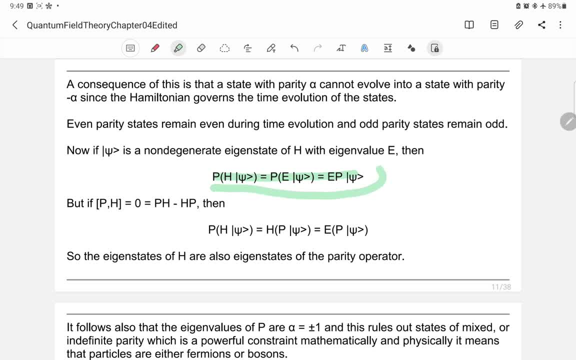 with eigenvalue e, then you you would have this. but if you have, uh, but if the hamiltonian and the parity operator is commutative, then you're gonna also have this. so they're just the same. so the eigenstates of h or hamiltonian are also eigenstates of the parity operator. 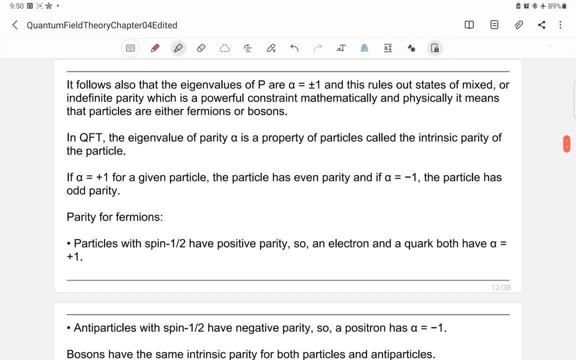 again earlier. the eigenvalues of b are positive, negative one, and this rules out states of mixed or indefinite parity. this is a powerful constraint. mathematically and physically, it implies that the particles are, or the wave function represents a fermion or a boson. if uh, 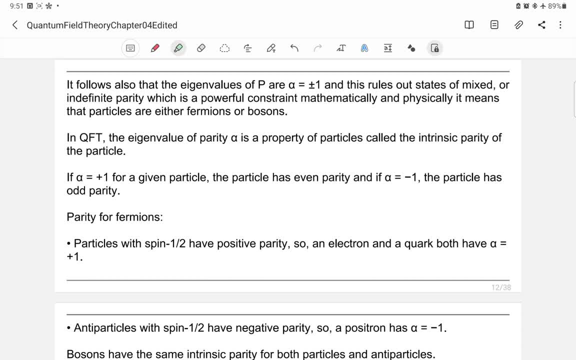 if the eigenvalue of parity is is positive one, then uh, for, for that particle or for that wave function that is representing the particle, uh, the parity is even, and if it is um negative one, the particle has odd parity. so in quantum field theory the eigenvalue of parity, alpha- is a property of particles called 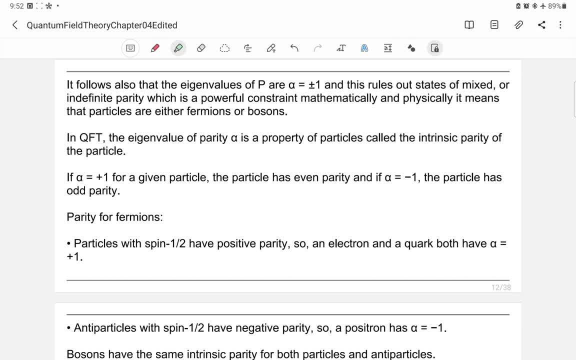 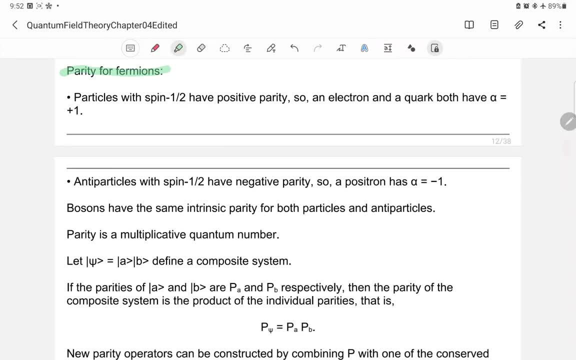 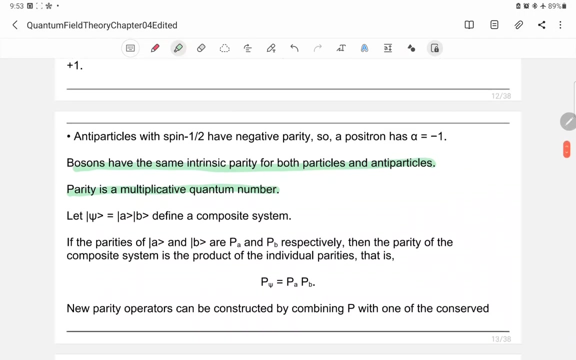 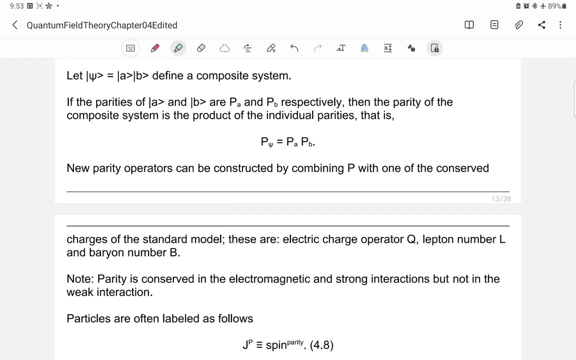 the intrinsic parity of that particle. so for fermions particles with spin, one half have positive parity. so an electron and a quark both have 荷. parity is a multiplicative quantum number. so let's look at this so if you have a composite system, so your wave function would be a product of 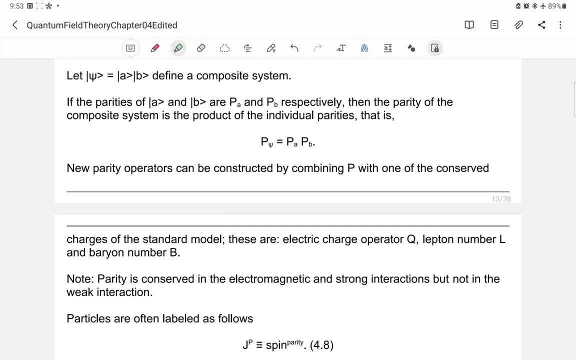 two wave functions composing the system. so, say your, your wave function is this one. so that defines a composite system. if the priorities of a and b are p a and p b respectively, then the parity of the composite system is the product of the individual priorities that compose the system. 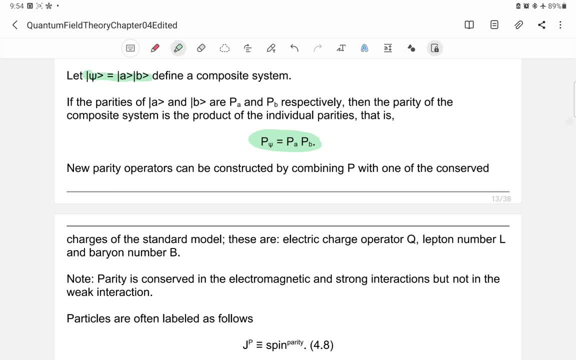 so the new parity operators can be constructed by combining p with one of the conserved charges of the standard model. these are electric charge operator q and lepton number and barrier number b. so we know all of these barrier number going back. these are the things to remember. 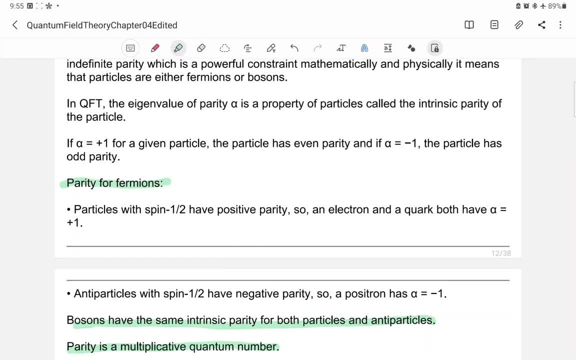 so for particles with spin, one half have positive parity. so an electric and a quark both have parity of positive one. remember that electron and quarks have parity of one. there are anti-particles, that means positron and anti-quarks have have negative parity. so these are the things that you should remember when dealing with. 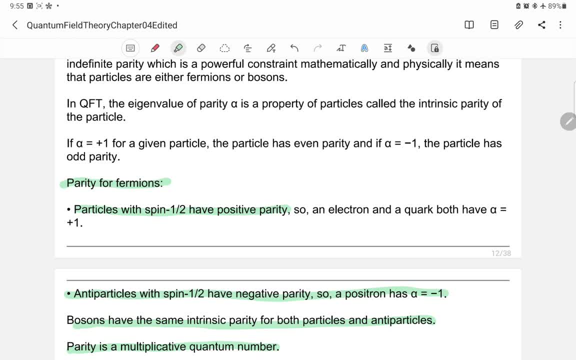 uh, particle interactions. you can check the priorities, for example. so when you have a, when you have a pi, particle or pion, so this is what this is composed of: a quark and an anti-quark. so the parity here is negative one in that case, because you have positive one and an anti-quark. so the parity here is: 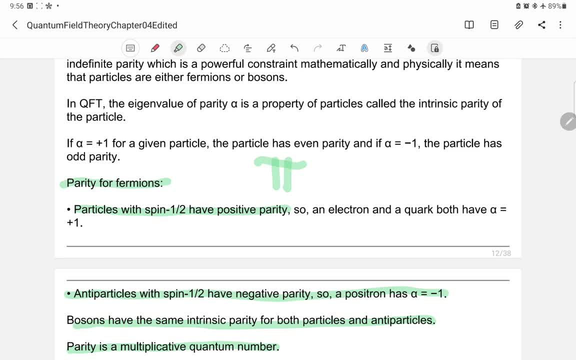 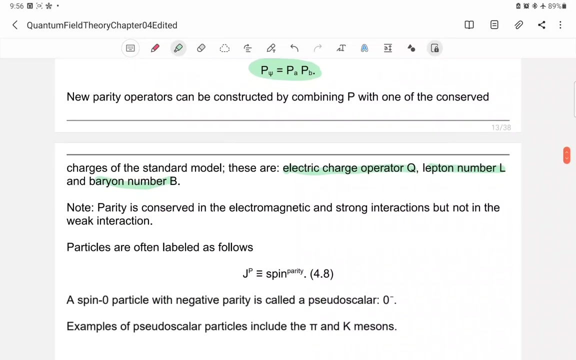 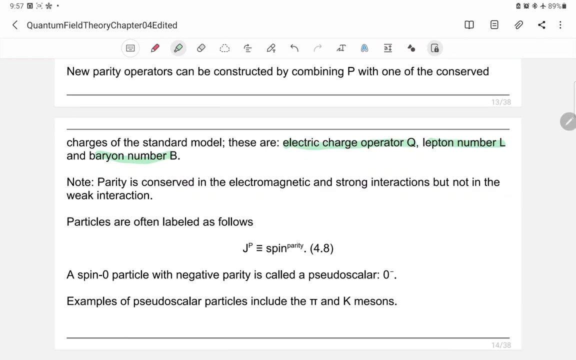 negative one in that case, because you have positive one and a negative one. so that is the priority of uh of a meson. so anyway, your electric charge operator Q is are just the charges of the particles and they are additive quantum numbers. left, the number L are just the number of leptons present in. 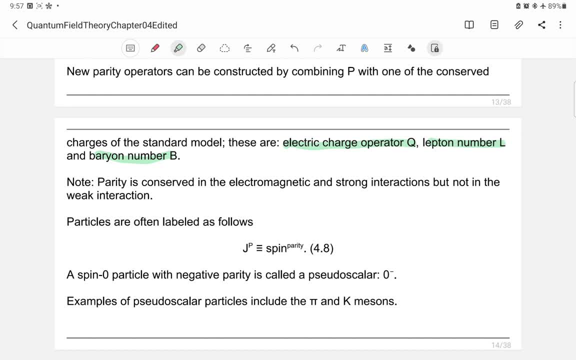 the interaction and that is supposed to be conserved, and thus the leptin number in the initial state should be the same in the final state, as well as the barrier number B. these are the number of variants involved in the interaction. now there's a very important, important note here: parity is conserved in. 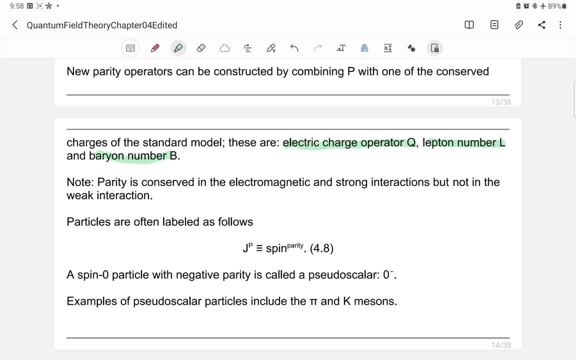 electromagnetic and strong interaction, but it is violated in weak interaction. so in in weak interaction you have a violation of parity. so in in weak interaction you have a violation of parity. by the way, there is a labeling of particles. here you have JP DJ, here we just be spinn and Party, and P we just be parity. 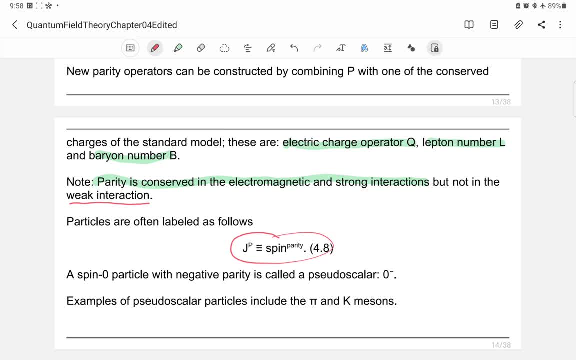 for up for a spin 0 particle with negative parity, that is a pseudo-scalar and they are represented by this JP labeling. so examples of pseudo scalar particles are pi and k meson. so, as I've said, they have parities of negative because they are quarks and anti-quarks. 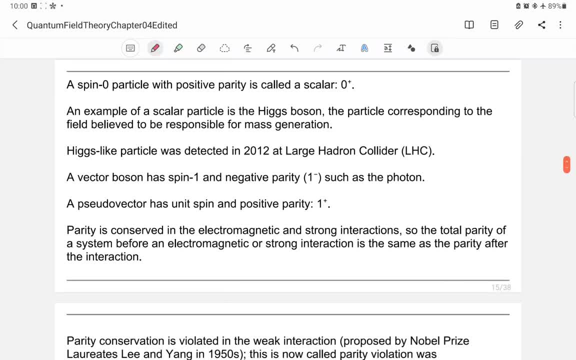 a spin zero- particle positive party is called a scalar, and it is labeled this way: spin zero- parity positive one. an example of a scalar particle is a, the Higgs boson, the particle corresponding to the field believed to be responsible for the mass generation of the gauge bosons. 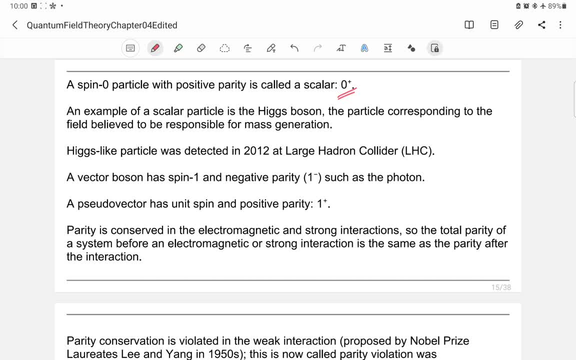 Higgs like particles, was detected in 2012 at the Large Hadron Collider. now you have a boson with spin one and their parity is negative, such as the photon, so it's labeled by this, and you have also a pseudo vector that has a unit spin spin. 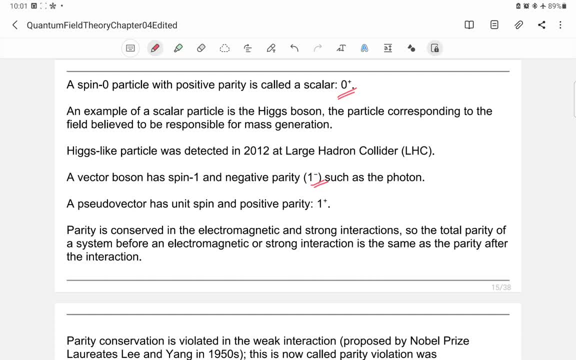 one and it's it's labeling would have to be one plus, because it has a parity, a positive parity. so, again, parity is conserved in electromagnetic and strong interaction. so initially, before the electromagnetic and strong interaction, the parity is is supposed to be the same with the 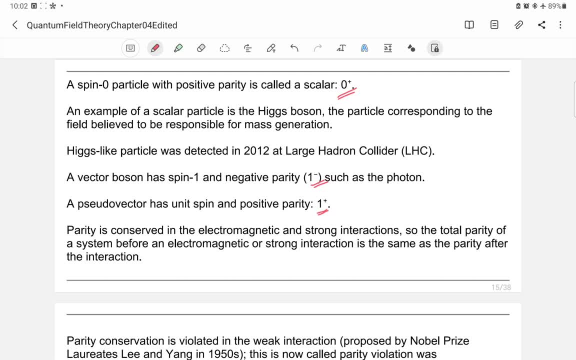 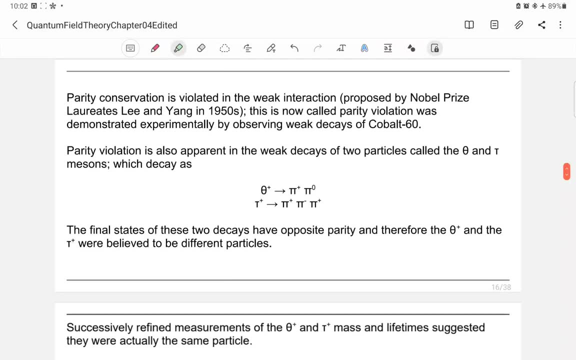 final parity of the system now probably is not conserved or violated in the weak interaction. this is proposed by a Nobel Prize laureates, Li and young in the nineteen fifties. this is now called a parity violation and can be demonstrated experimentally by observing weak decays of cobalt-60. 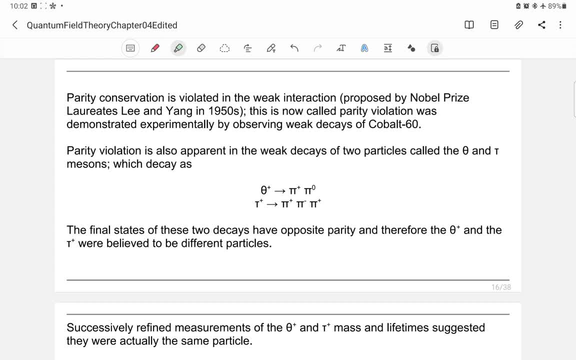 Parity violation is also apparent in the weak decays of two particles, Theta and Tau mesons. They decay in this particular decay. So here you have a meson which is negative one on the left side, and on the right side you have different parities. 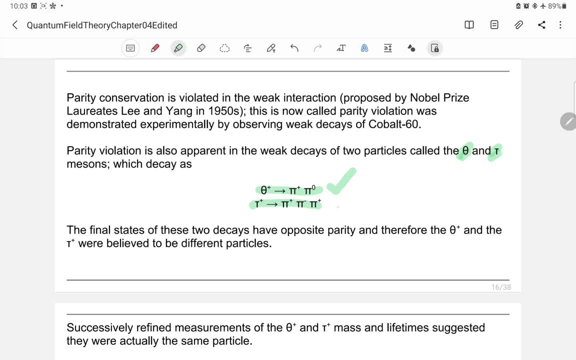 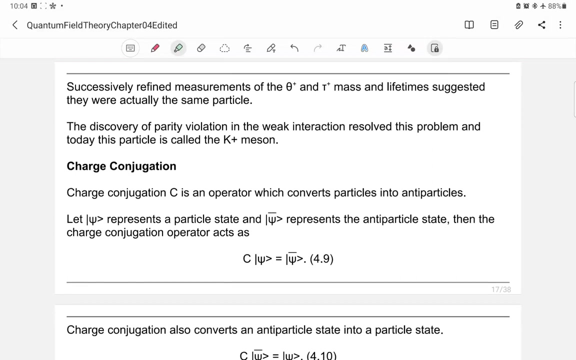 This one is positive one and this one is negative one. The final states of this These two decays have opposite parity and therefore Theta plus and Tau plus were believed to be different particles, but refined measurements show that they are actually the same particle And at this moment these particles are now called K plus meson. 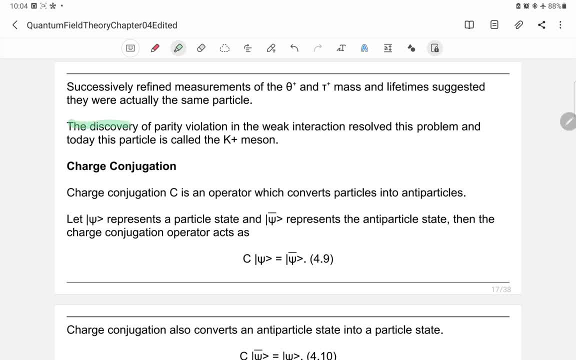 So the discovery of parity violation in the weak interaction resolved this problem and today this call the K plus meson. So let's move on and we'll be able to see how the violation, how this parity violation is manifested in the weak interaction. Another discrete symmetry is what we call the charge conjugation. 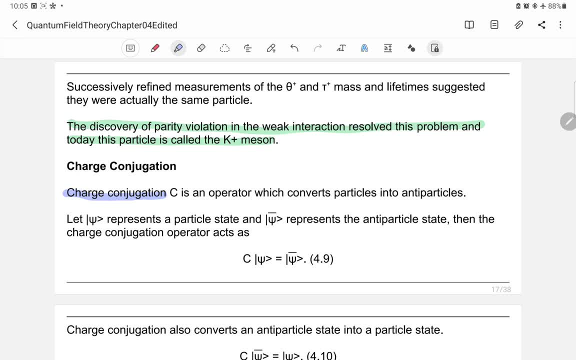 Charge conjugation denoted by C is an operator which converts particles into antiparticles. When the state psi represents a particle state and state psi bar represents an antiparticle state, then the charge conjugation operator acts as this one here, So it converts your particle into an antiparticle. 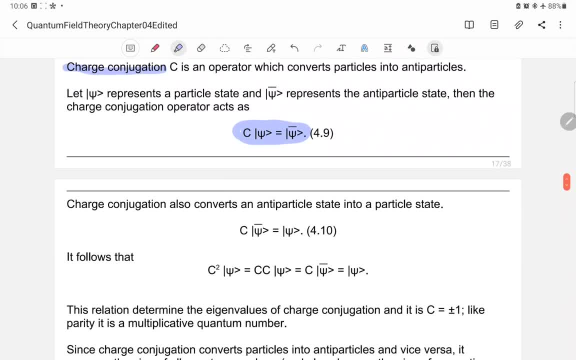 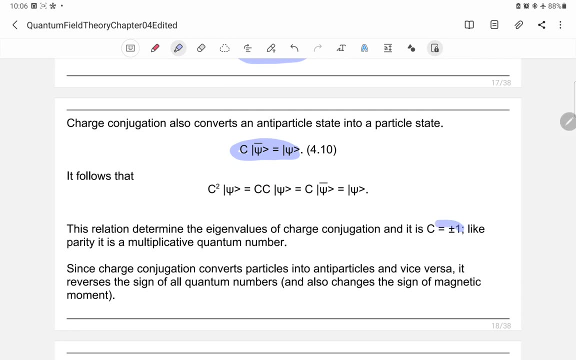 But if C also acts on an antiparticle, it will convert it to a particle, like here. So it follows also that the C has eigenvalues of 1 plus. I mean plus minus 1. Because if you operate two charge, two successive charge conjugation, it will go back to the 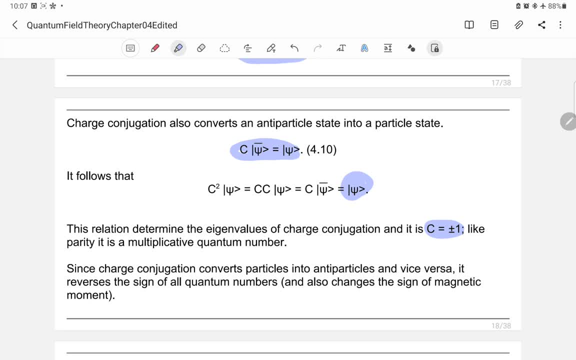 same state psi. And also charge conjugation is a particle, It is a multiplicative quantum number- Now this important note here, if you're really serious about particle physics. So charge conjugation converts particles into antiparticles and vice versa. 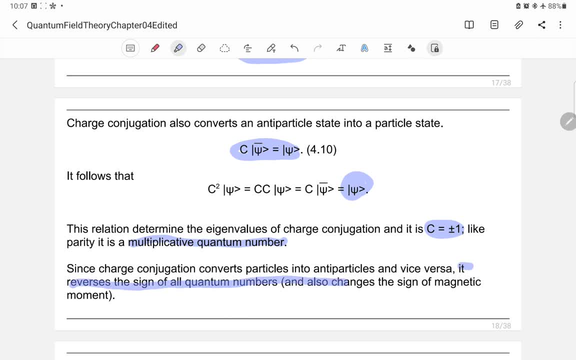 It also reverses the sign of all of its quantum numbers and also changes the sign of the magnetic moment. Okay, That is very important to remember when you do charge conjugation. So everything reverses all quantum numbers, including the sign of the magnetic moment. 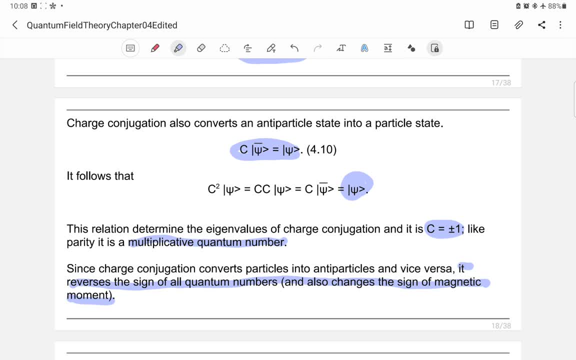 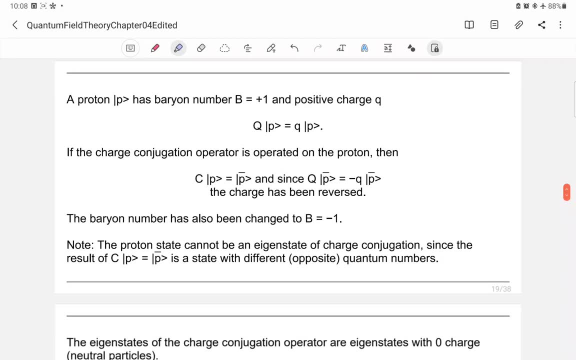 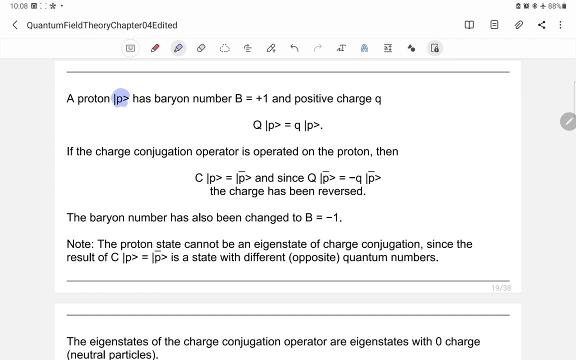 of the particle. To illustrate that, The proton P here has a barren number equal to positive 1, because it is a particle, And the positive charge Q. So QP is the charge operator here. It gives you the charge of the proton Q. 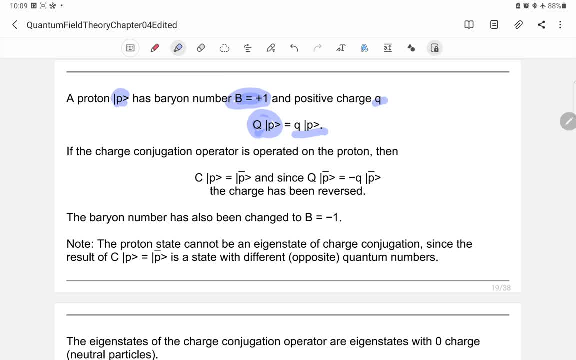 If the charge conjugation operator is operated on the proton, then your proton becomes an antiproton And since your Q is positive, P here equals the charge to the proton times P- your Q of anti-proton will give you a negative Q. So the charge has been reversed and then also the barium number is changed to a negative one. Everything, all of the quantum numbers, are supposed to have an opposite sign. if you do charge conjugation operator, 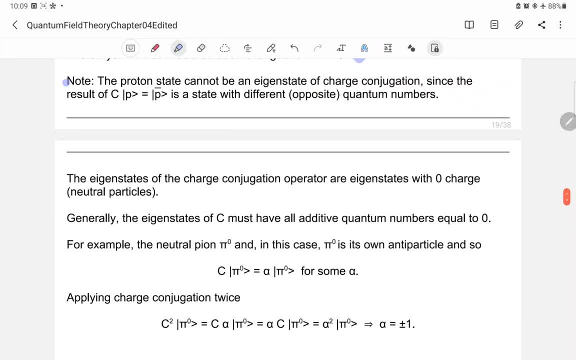 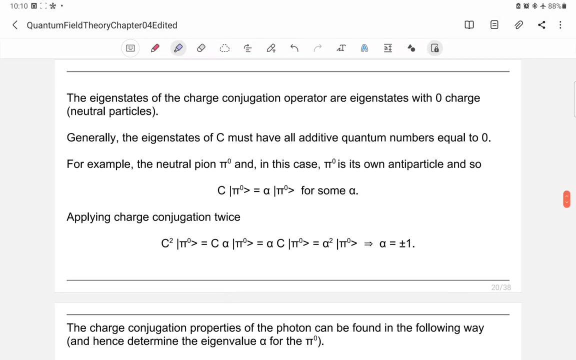 Now, the proton state cannot be an eigenstate of charge conjugation, since the result of this operation is a state with different or opposite quantum numbers. This is also important. The eigenstate, The eigenstates of the charge conjugation operator are eigenstates with zero charge neutral particles. 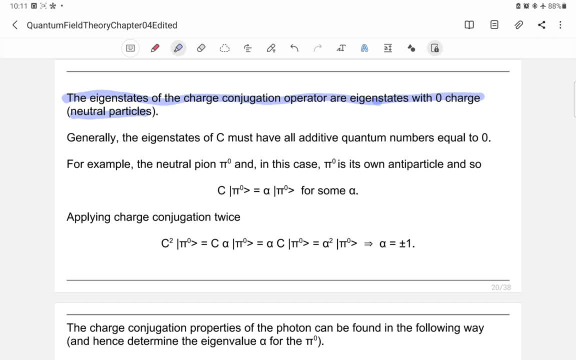 So in this particular case you have a pion, So the pion, the neutral pion I mean, because you have three pions: pi plus, pi minus and pi zero. In this case, if you're doing an operation, applied to the pion. 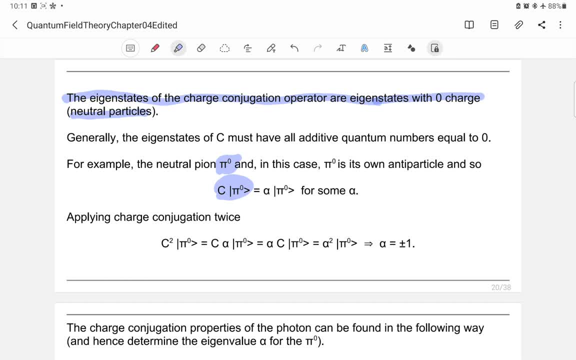 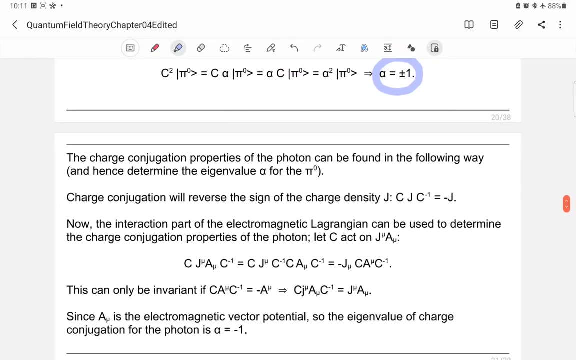 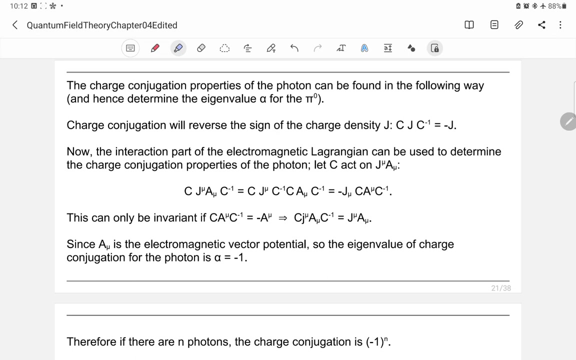 That is a charge conjugation, and it also gives you the same particle, because it's an antiparticle of itself, And so in this particular case, your alpha is equal to positive negative one, But for a particle called photon it's a particle of light. 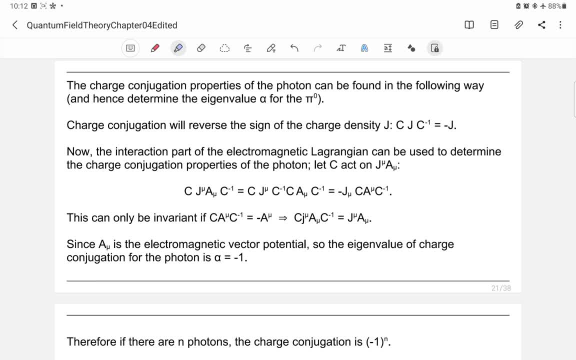 The charge conjugation property is a little bit tricky but we can follow this process here and we'll be able to get how the charge conjugation goes with production of photon Photons in an interaction, So charge conjugation will reverse the sign of the charge density. 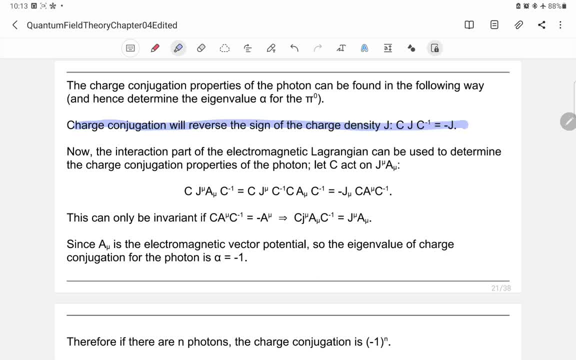 So here you have, Or the current I mean. So if you apply this charge conjugation on the current density, So it will give you negative J. So now the interaction part of the electromagnetic Lagrangian can be used to determine the charge conjugation properties of the photon. 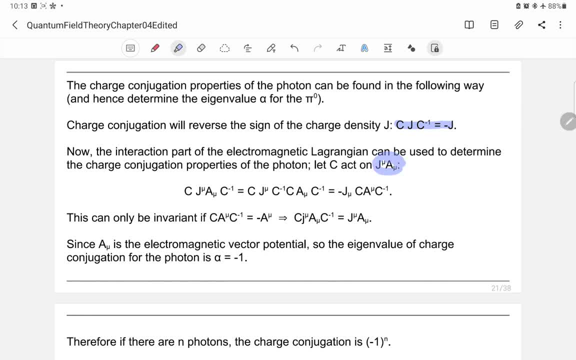 Let's see act on this one: The field A representing the photon, and then you have the current density. So if you apply that, You can- actually this is just an identity- so you can do that, You can put that in between or anywhere in the expression, so that you will have this one here and this is just equal to negative J mu. 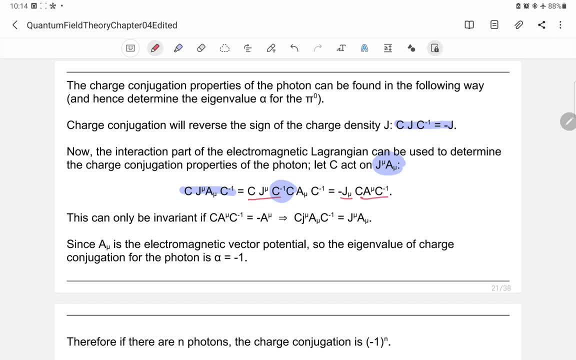 And this one is, of course, your conjugation of your Field, the field representing the photon, and that can only be invariant. when you have this and if you have a negative A mu there, you'll be able to achieve invariance. 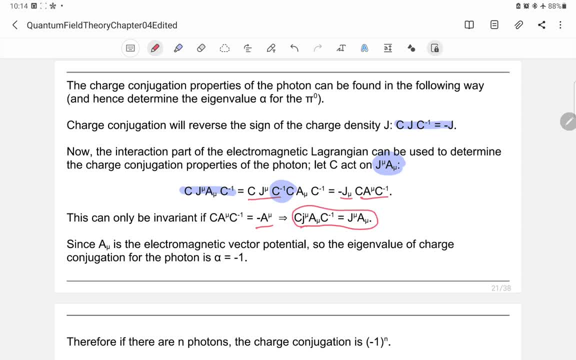 Here Now, since A mu is the electromagnetic vector potential, so the eigenvalue of charge conjugation for the photon is alpha equals negative one. So if there are N photons produced in an interaction, the charge conjugation is just equal to negative one raised to the number of photons produced. 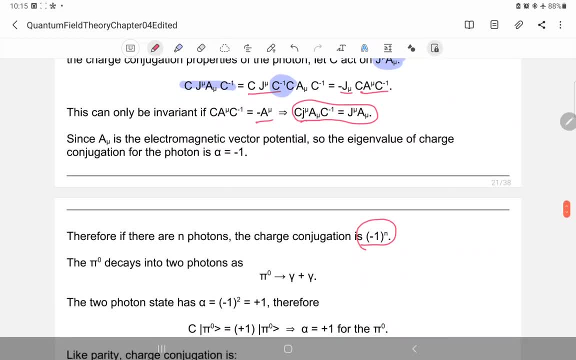 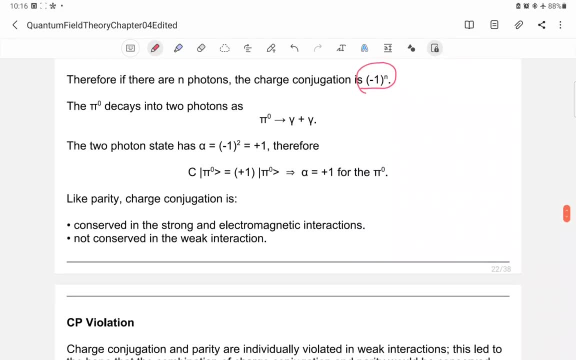 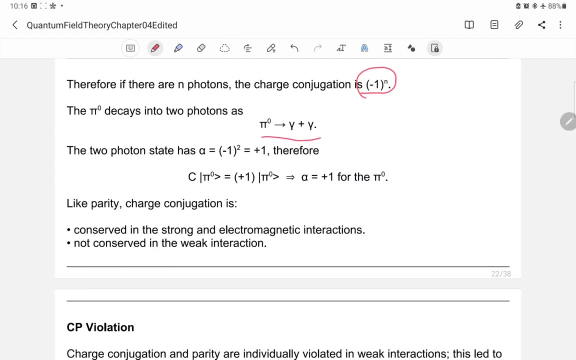 So in this case, if you have a neutral pion decaying into two photons, then the two photon state has an alpha equal to negative one squared, which is positive one. And in this case If you apply charge conjugation on neutral pion, then you will have to get a positive one because of this one, this rule I mean. 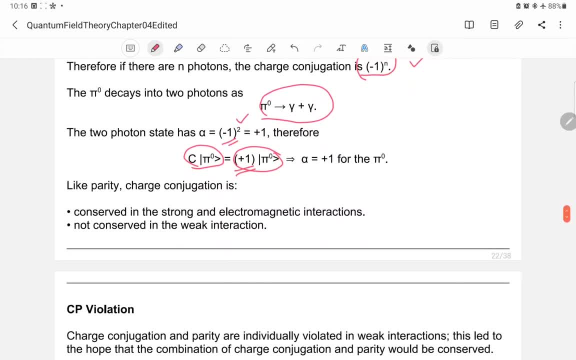 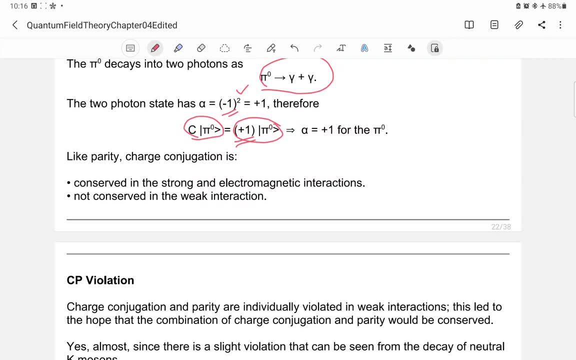 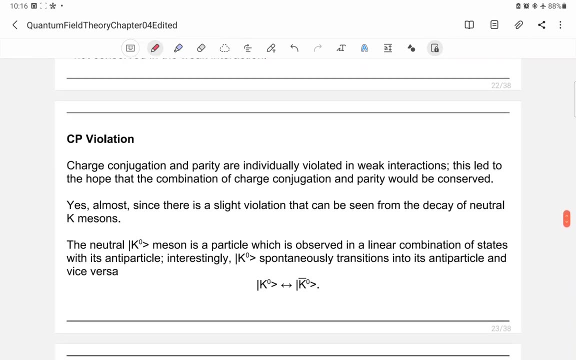 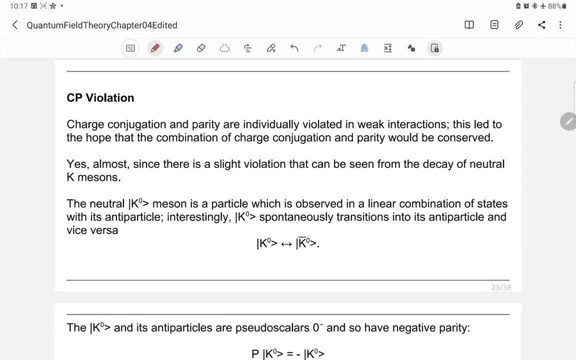 Yeah, this rule, So like parity, charge conjugation is conserved in strong and electromagnetic Interaction, but not really in electric interaction. Let's look at that in the following sections. Now let's talk about CP violation. This is the product of charge conjugation, and 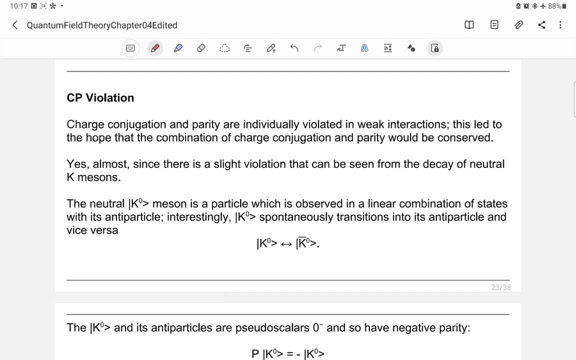 Parity, Charge conjugation and parity are violated, each violated in weak interactions, And this led to the hope that the combination of Charge conjugation and parity would be conserved in weak interactions. And the answer is yes, Almost, Because there is a slight violation. 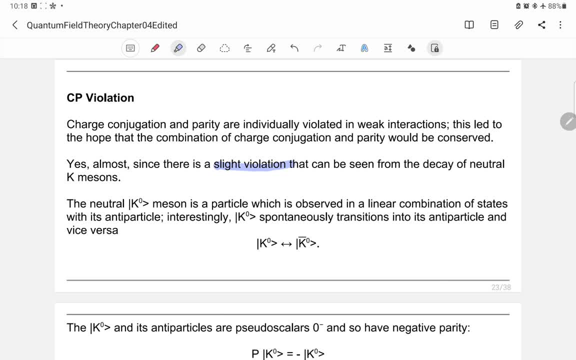 That can be seen from the decay of a neutral, neutral, neutral k meson. The neutral k meson state Is a particle which is observed in a linear combination of states, With its antiparticle And, interestingly, k, zero state or neutral. 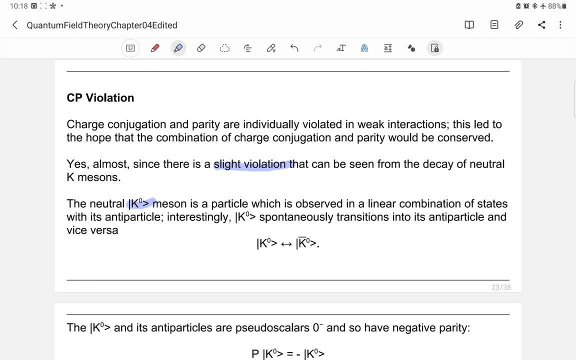 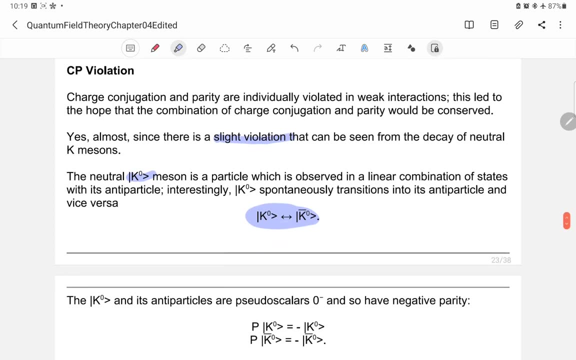 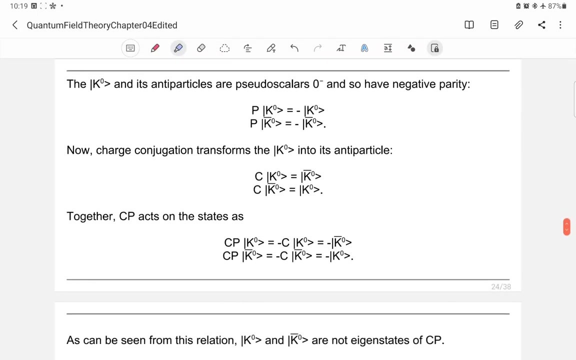 K meson Spoon Spontaneously transition into its antiparticle and vice versa. So this is the behavior of the K meson: It oscillates into an antiparticle And Back to itself. Now your, Your k meson is: 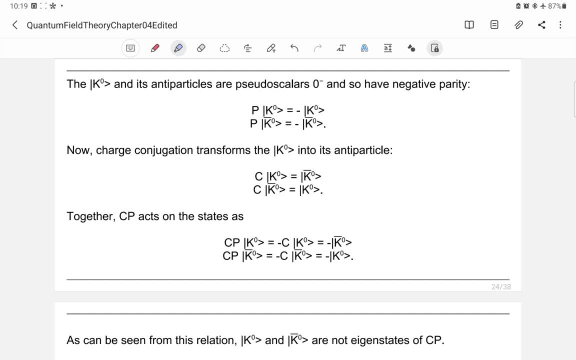 Pseudostolar, So it has spin zero and it's Of course Its parity is negative. So if you Operate P on k zero, It will give you a negative K Zero. And then For The antiparticle, 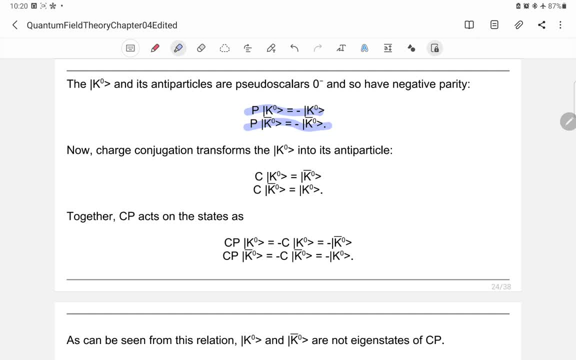 The k meson. It will also give you a negative Eigen value. Now let's Let's look at the charge conjugation Of k, Neutral K meson state. So if you Do this, It will convert into an antiparticle. 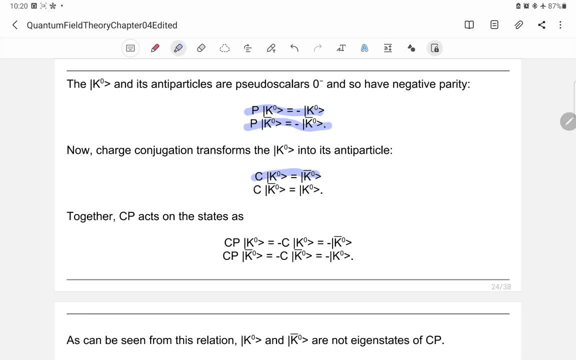 Or an anti k meson Neutral, And of course This one also Would be Would result. So together You can See from here That Cp Together Acting on On K Gives you An antiparticle. 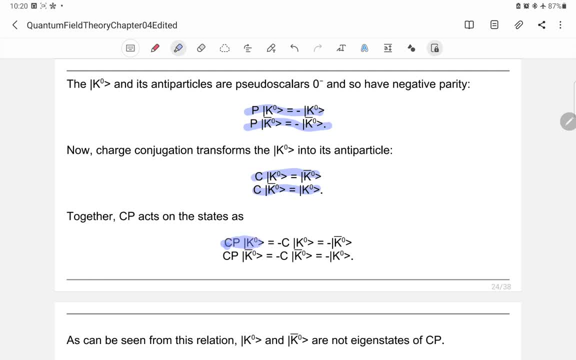 And With A Negative Parity. So You can See That Cp Together Acting On On, And This One Here Is Also Giving You A Particle For. 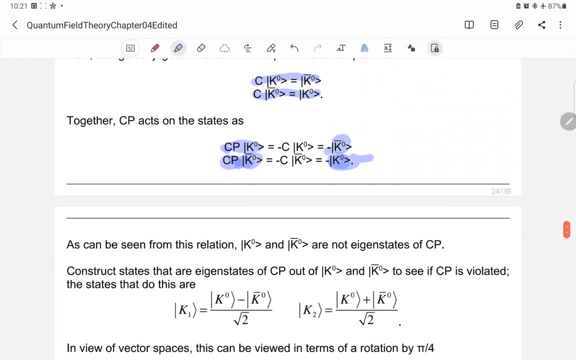 An Antiparticle, Giving You An Antiparticle With A Negative Parity, As Can Be Seen From This Relation K? M. Earlier They Constructed States. 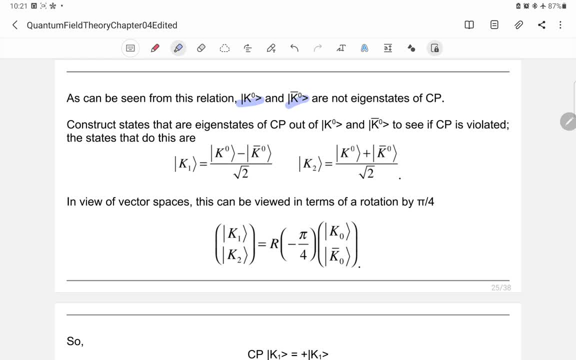 That Are Eigenstates Of Cp Out Of K O And K O Bar Or The Antiparticle, And Check If They, If Cp Is Still. 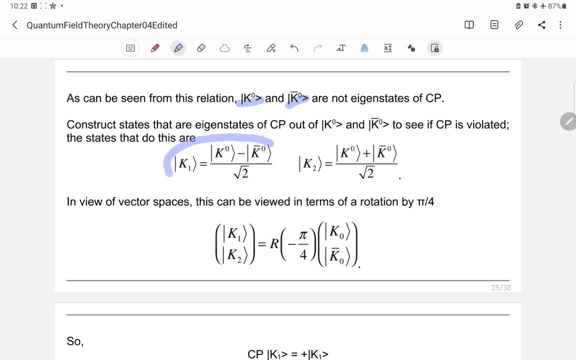 Between K Zero And K Bar. This One Will They Call K One And K Two. Normalized Combinations Of The Two Part The Of The. 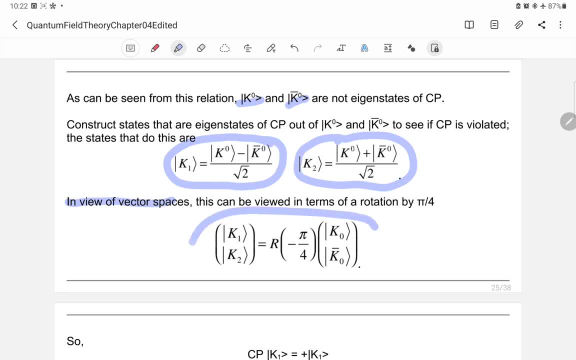 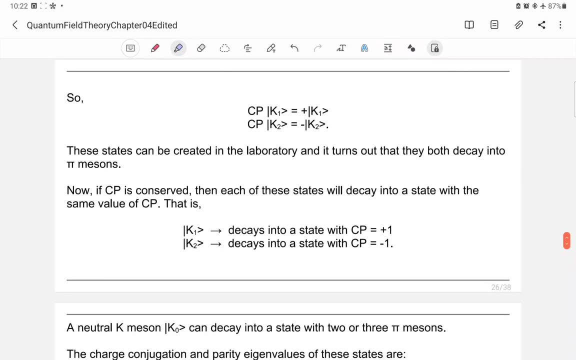 K Meson And The Anti, These Two Into This One. Now You Can See That They Are Eigenstates Of Cp, Because It Is Now K. 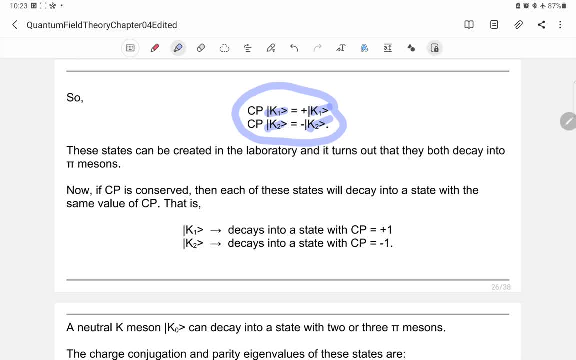 In The Laboratory, It Turns Out That K One And K Two Both Decay Into Pie Mesons. Now, In This Case, Since You Have K, 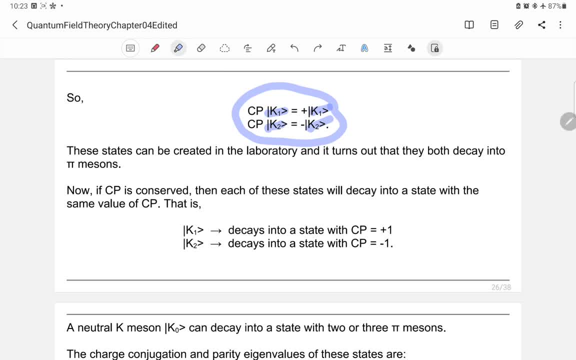 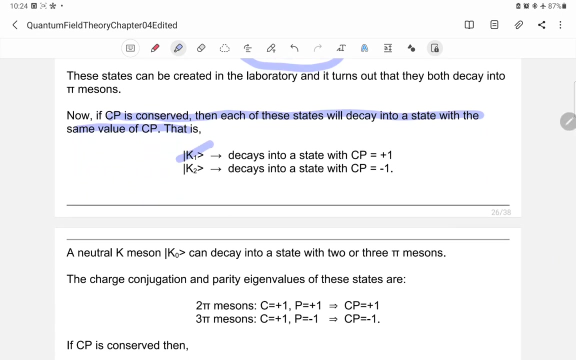 One Here And K Is Now Conserved, So Cp Is Conserved. Then Each Of These States Will Decay Into A State With The Same Value. 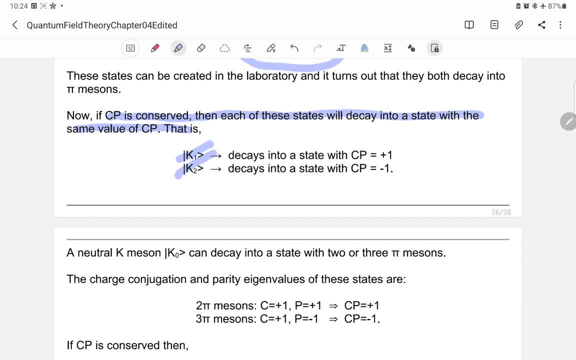 Of Cp, That Is Your, A Neutral K Meson. K Can Decay Into A State With Two Or Three Pie Mesons, So The Charge Conjugation. 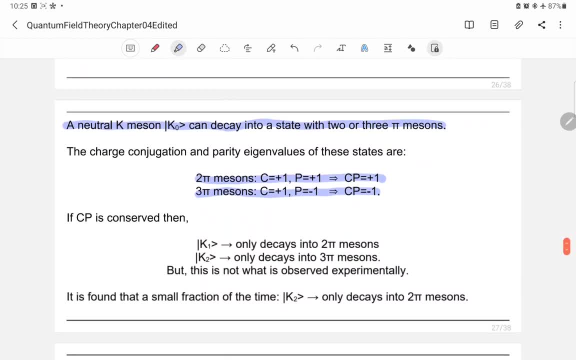 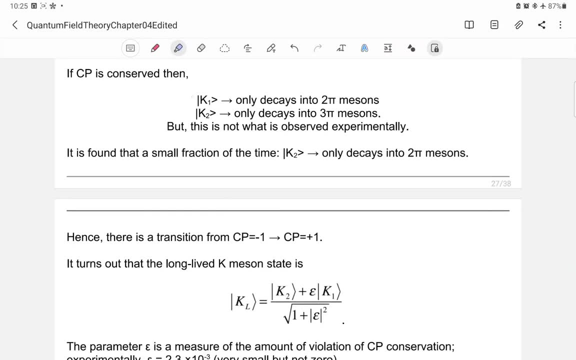 Party I can Balance Of These States Are This One K One Only Decays Into Two Pie Mesons. And If, If Cp Is Also Conserved. 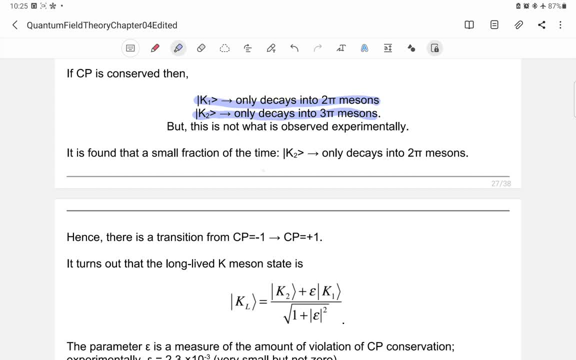 Keto Would Only Decay Into Three Pie Mesons, But Experimentally This Is Not That A Small Fraction Of The Time K2. Decays In Only 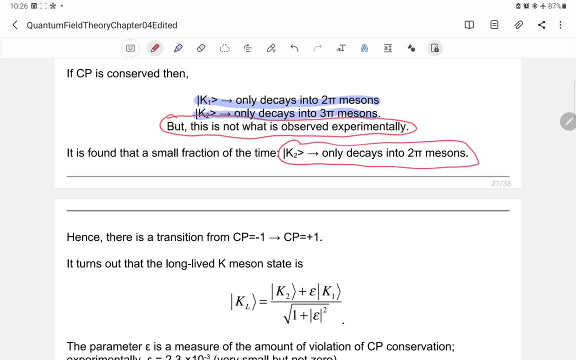 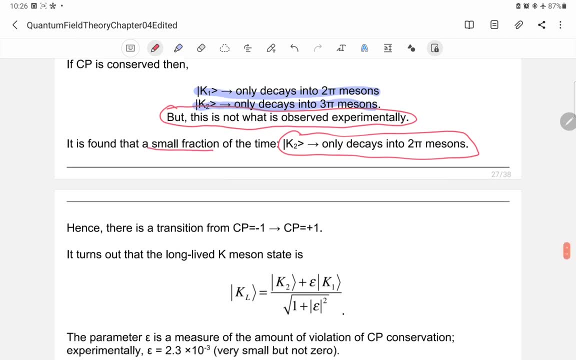 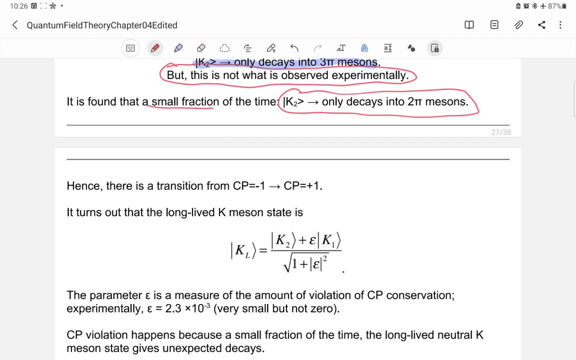 Two Pie Mesons. So There's A Slight Violation Of The Cp, Although It's Just A Very Small Fraction. Hence K1.. So It Turns: 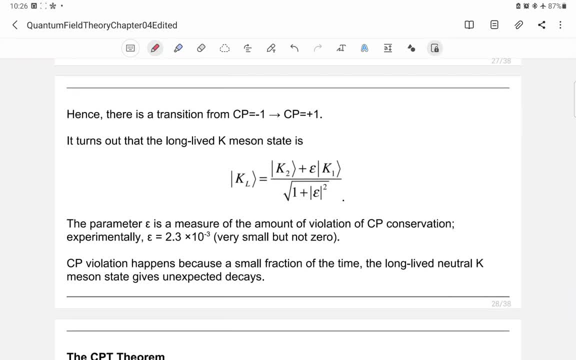 Out That That's A Particle Called Long Live K Meson State And This Is The Combination Of Kl From K1. And K2. K1.. 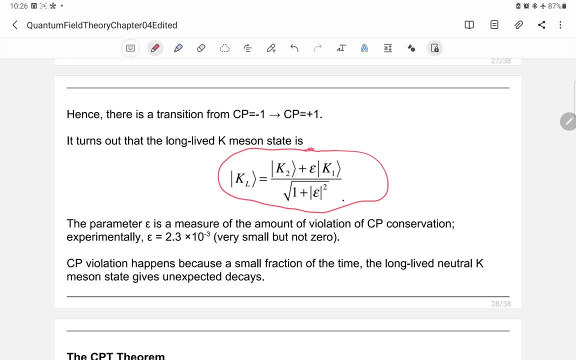 Is A Combination Of K1. And K2. With Some Coefficient Or Parameter, Here Epsilon, But This Epsilon Is Found To Be Very Small. 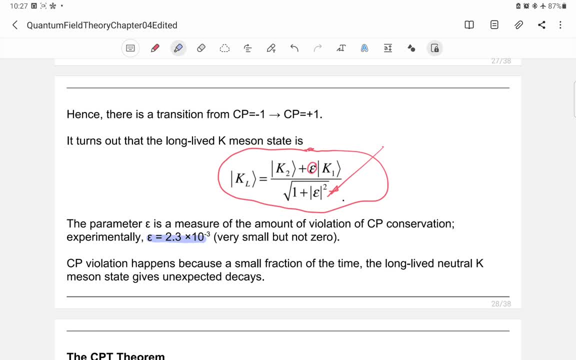 Experimentally. That's Just 2. Times, 10. To Negative 3. Time. So C B Is Supposed To Be Conserved, But It Happens The 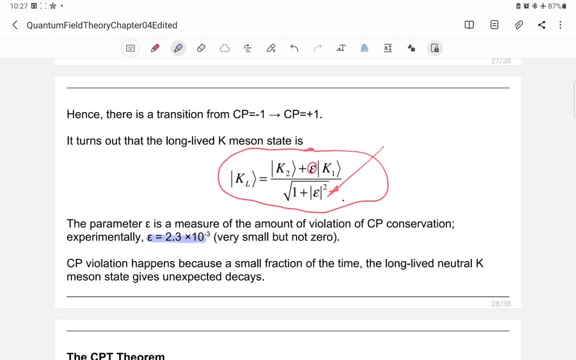 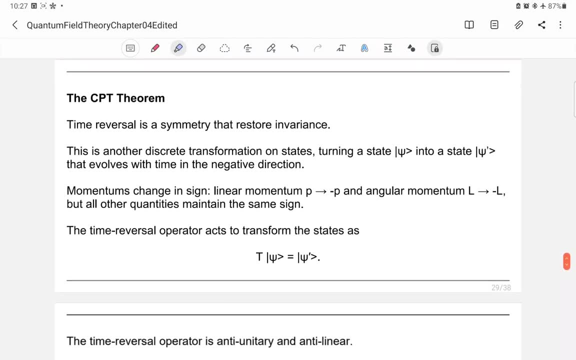 Violation Happens At A Small Fraction Of Time. That's What You Call C B- Violation In Variance, And We're Talking About That Restores. 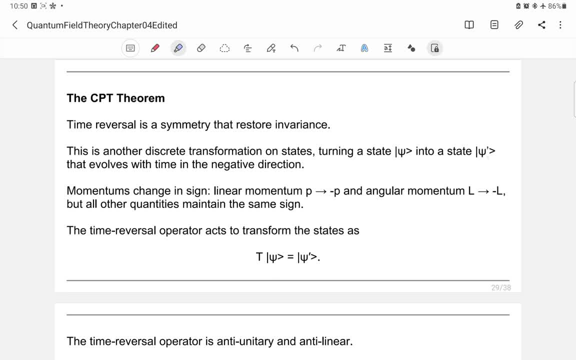 In Variance. This Is Another Discrete Transformation On States Turning A State Psi Into A Psi Prime. That Involves With Time In All Other. 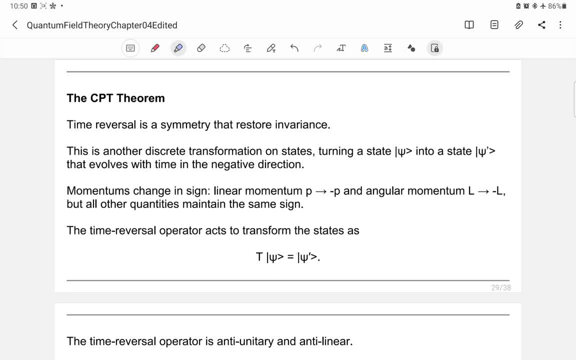 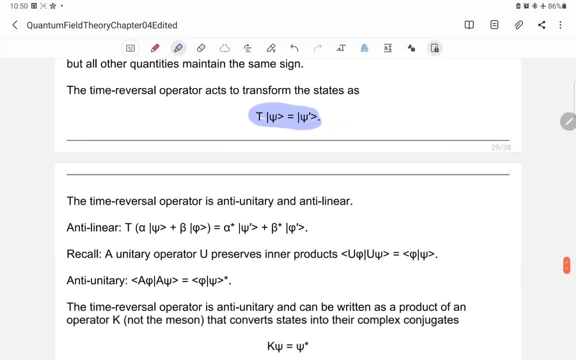 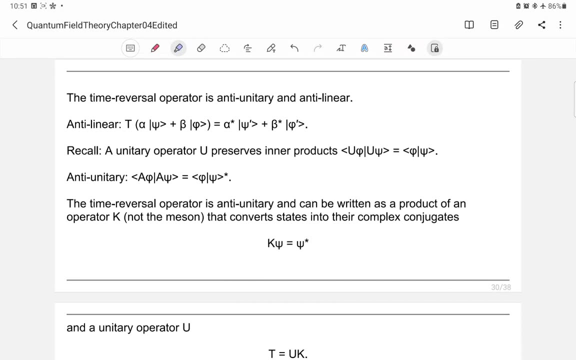 Quantities Maintain Same Sign, So This Is How It Transforms Time Reversal Operator Is An Anti Unitary And Anti Linear Operator. What I 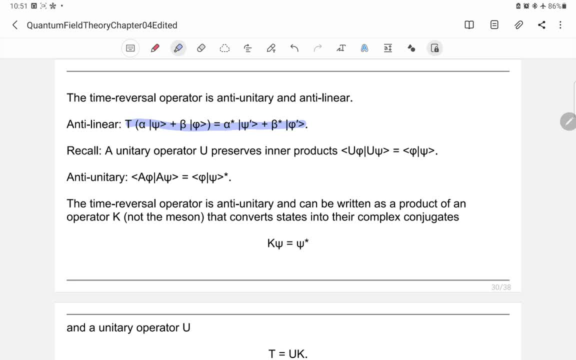 Mean With Anti Linear Is The Time Reversal Operator. It Gives You The Conjugate, The Conjugate And The State, The Prime State, And 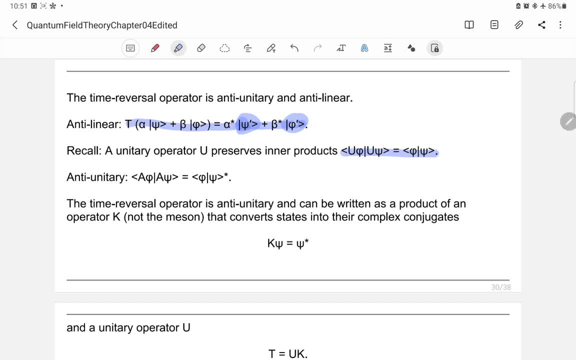 It's Also An Anti Unitary Because, Instead Of Preserving The Inner Product, This Means That The Inner Product Is The Conjugate, Not The 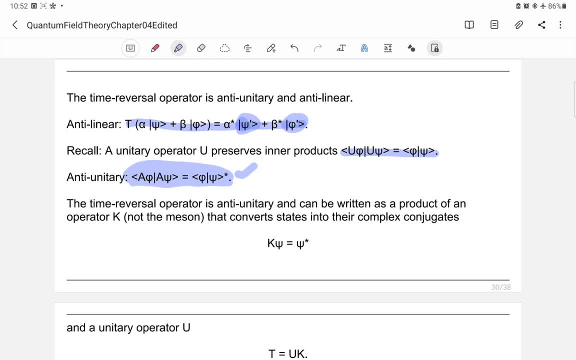 Original Inner Product. If You Apply That, I Mean If You Apply Time Reversal, So The Time Reversal Is Conjugates, So You Have. 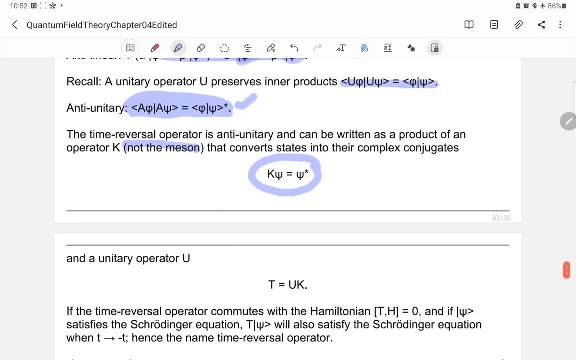 This One, And This Is The Operator K And A Unitary Operator U. This Is This One, And So Your Time Reversal Operator Is. 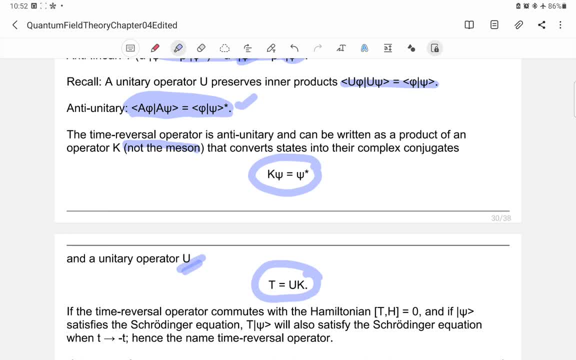 Gives You The Complex Conjugate. If The Time Reversal Operator Commutes With The Hamiltonian This One, And If Your Size Satisfies The 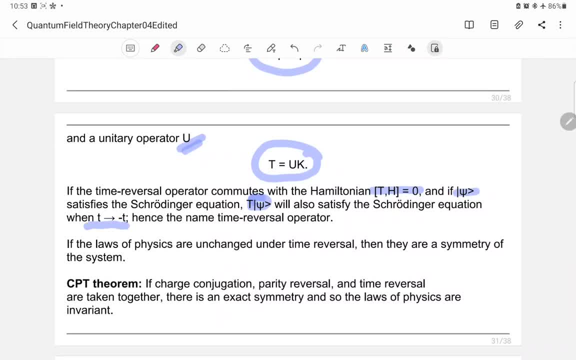 Schrodinger Equation, This Will Also Satisfy The Time Reversal Operator. If The Laws Of Physics Are Unchanged Under Time Reversal, Then 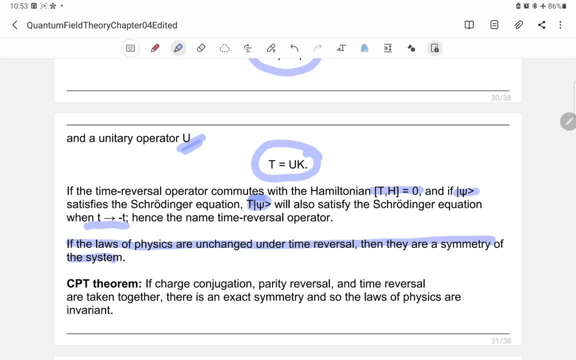 They Are A Symmetry Of The System. Now Here Is The C P T Theorem. So If Charge, Conjugation, Parity, Reversal And 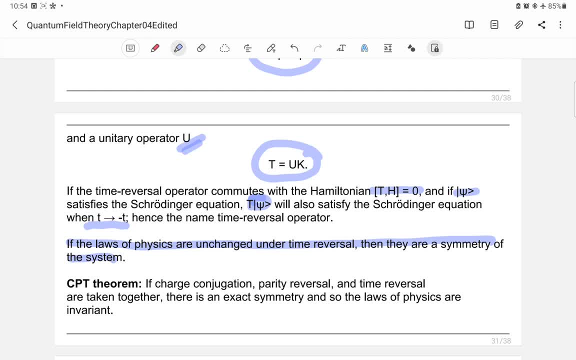 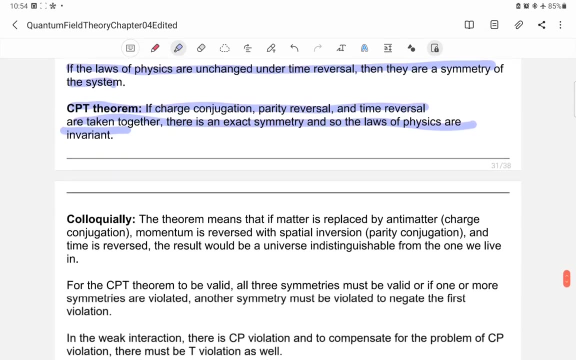 Time, Reversal Are Taken Together, There Is An Exact Symmetry. So The Laws Of Physics, So That The Laws Of Physics Are Invariant Place. 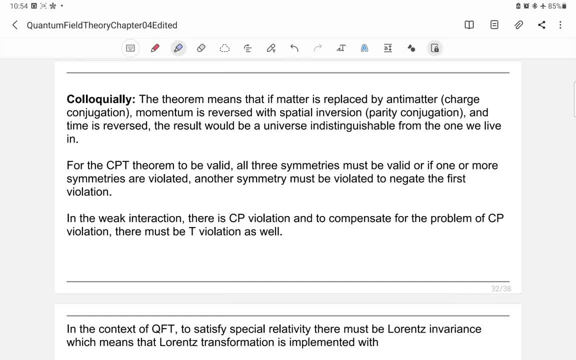 By Antimatter, That Is Charge Conjugation. Momentum Is Reversed With Spatial Inversion, That Is Parity Conjugation, And Time Is Reversed. The 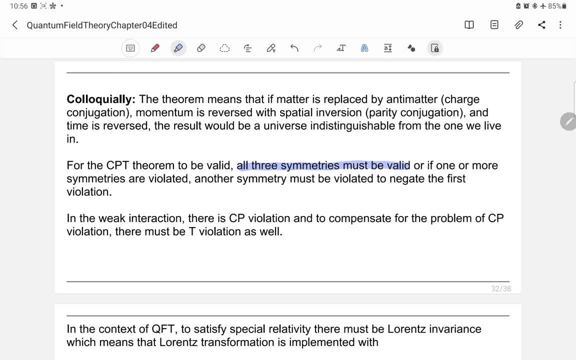 Result Would Be A Universe Indistinguishable From Another. Symmetry Would Have To Be Violated To Negate The First Violation. So This Is The 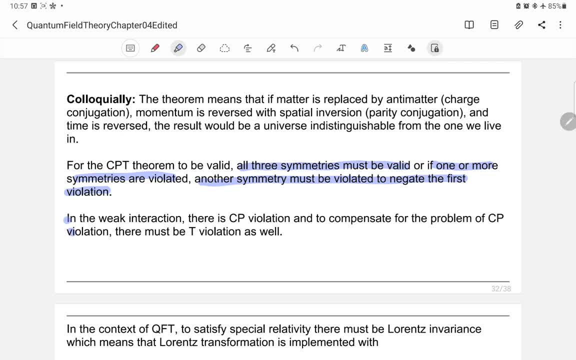 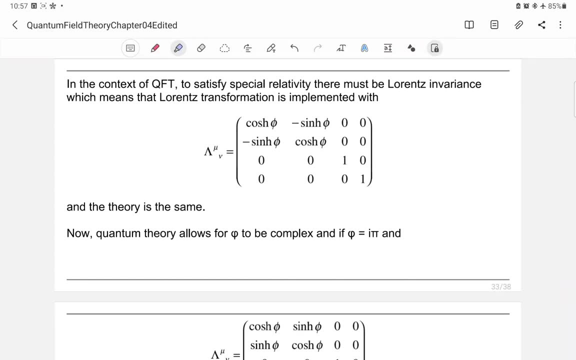 CPT Theorem: In The Weak Interaction There Is CP Violation To Compensate For. In Quantum Wheel Theory In The Context Of Quantum Wheel. 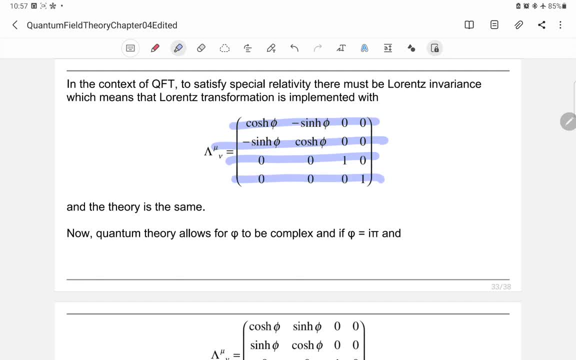 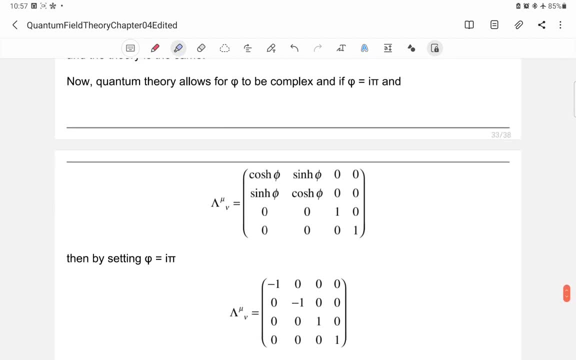 Theory. To Satisfy Special Relativity There Must Be Lorentz Environment, Which Means That Lorentz Transformation Is Implemented This Way, Your Transformation Would. 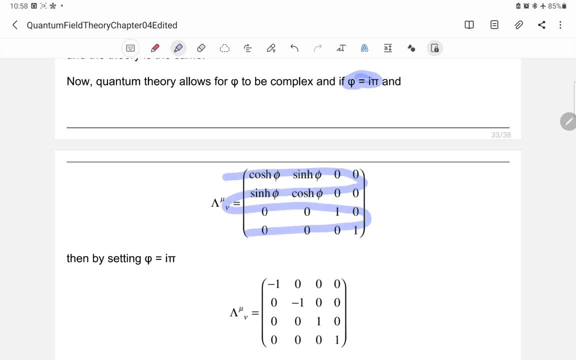 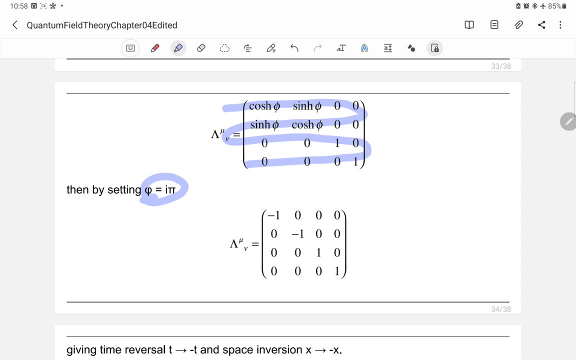 Be This. So By Setting Your Phi To Be This One And Then Putting It Into The Transformation Here, You Will Get This And This. So 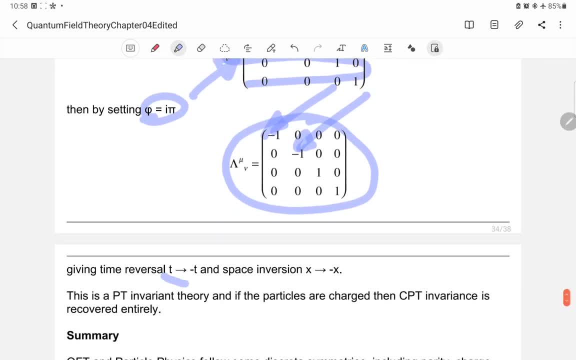 Giving Time. Reversal T. I Mean T Transforming Into Negative, And Space Inversion X Transforming Into Negative X. This Is Clearly A Parity.